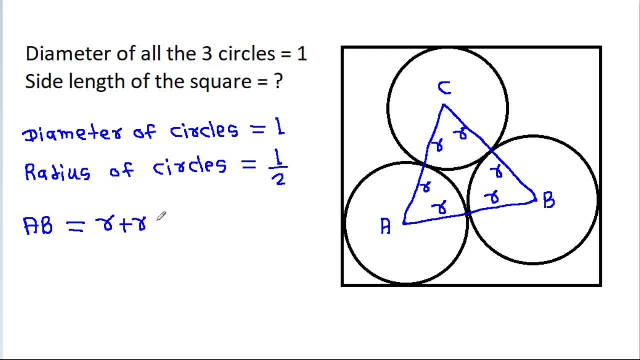 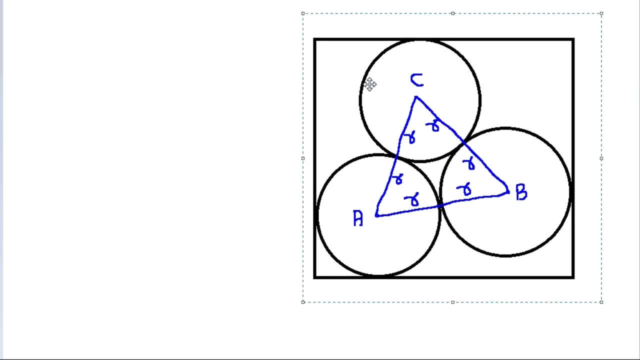 it will be R plus R, that is 2R, and it is 2 times 1 by 2, that will be 1. so BC will be 1 and CA will be 1, and suppose d square is P, Q, R, S and if we draw W X perpendicular to PS & W X, 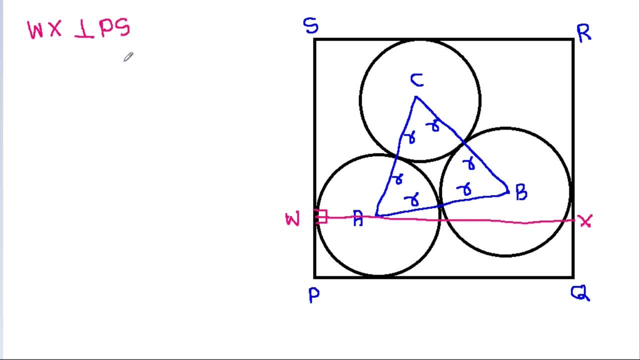 equalsFOC количество. but we will draw Mexico perpendicular to P and suppose this point is M, then W. it will be equal to WA – AM – MX And W it is equal to WA is radius – AM. if this angle is theta. 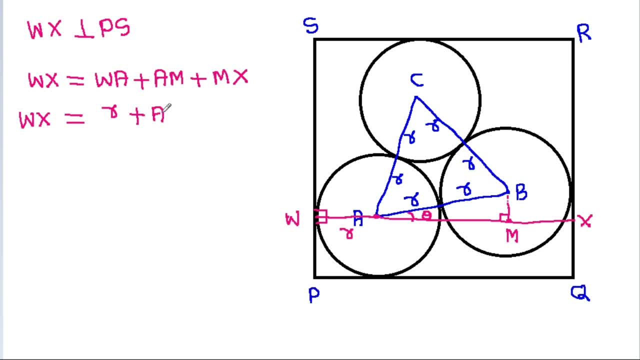 then AM is will be ab cos theta plus and mx will be equal to dissonant. that is radius, mx is radius and wx is equal to 1 by 2 plus ab is 1 times cos theta plus radius is 1 by 2, so wx is 1. 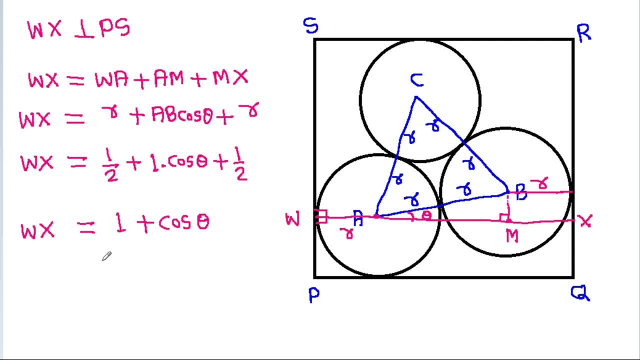 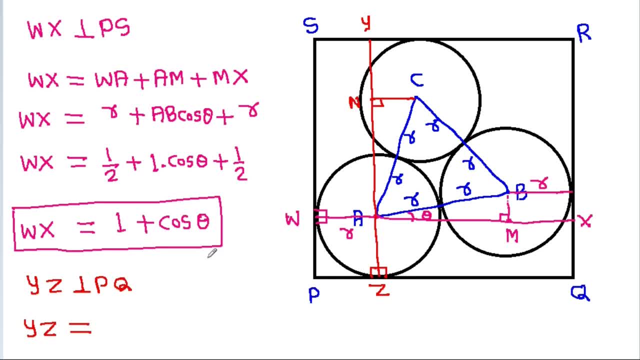 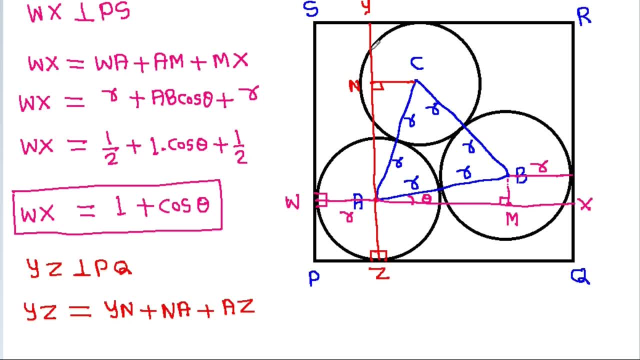 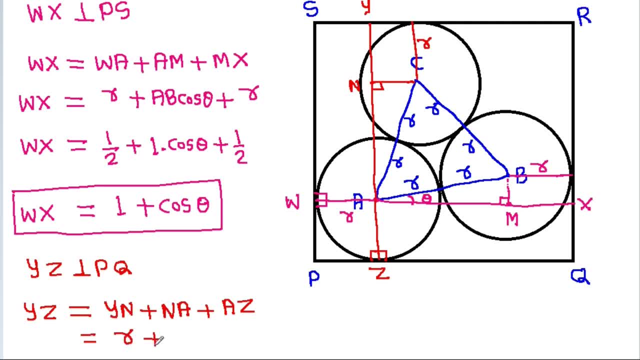 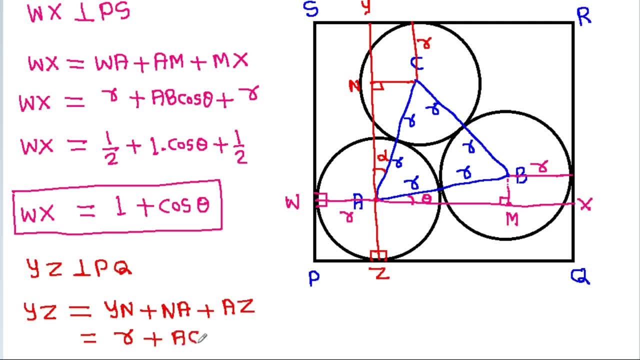 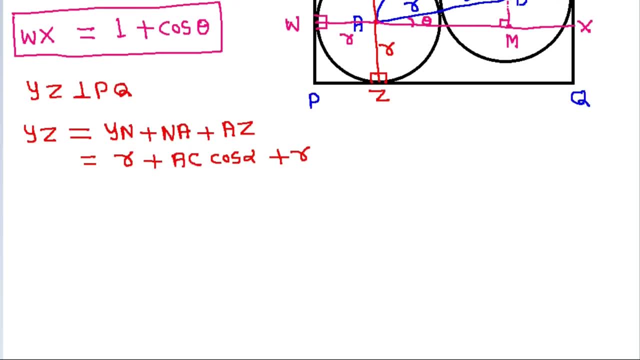 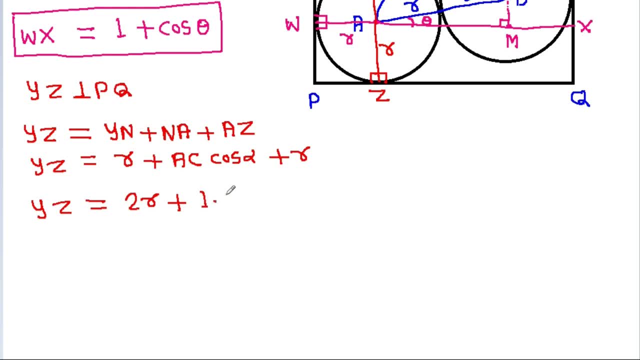 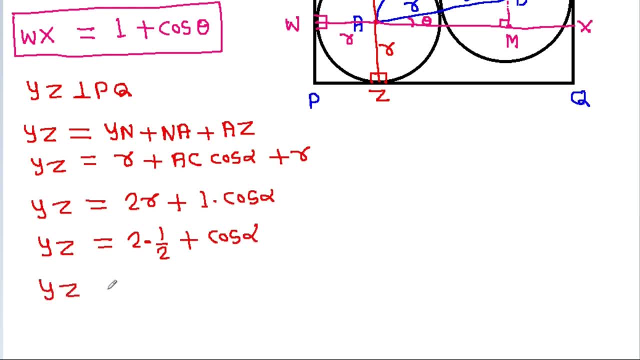 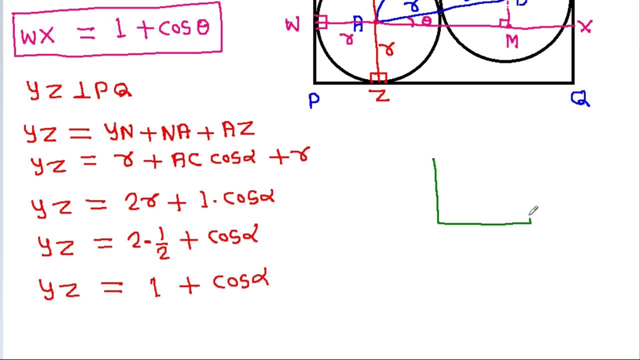 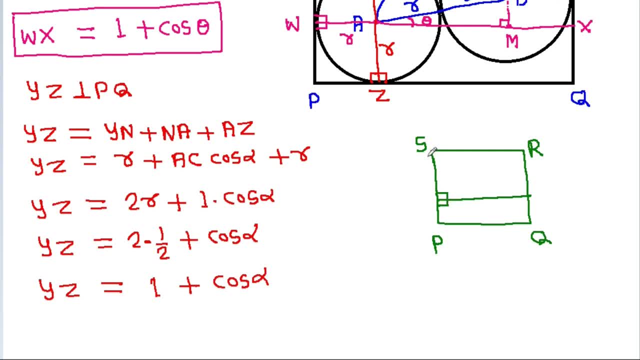 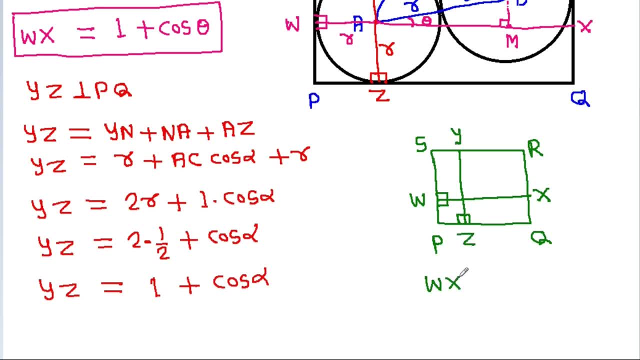 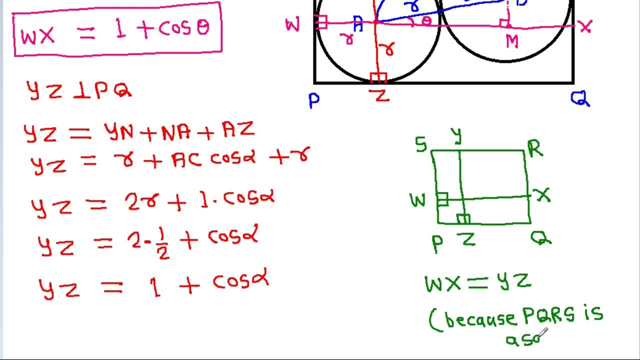 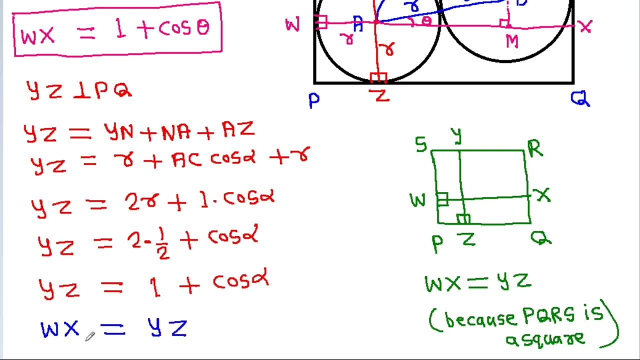 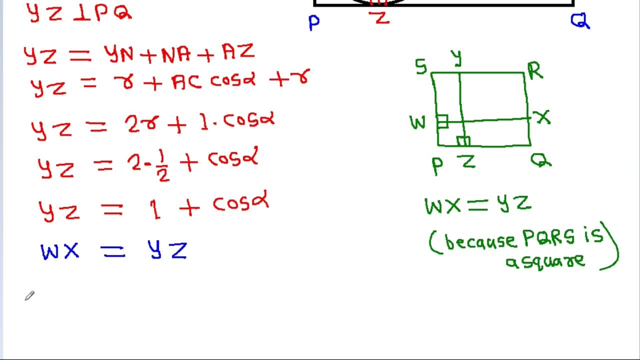 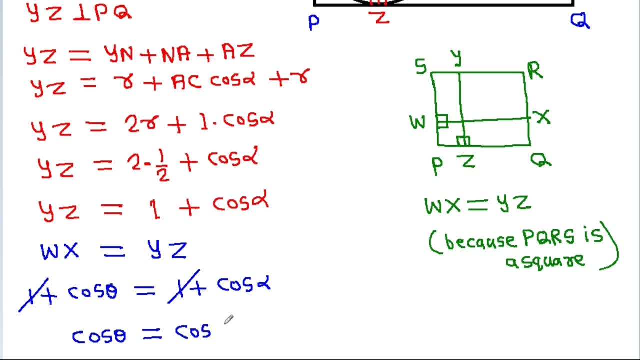 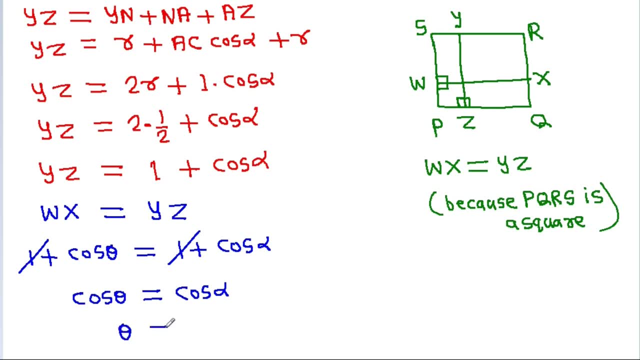 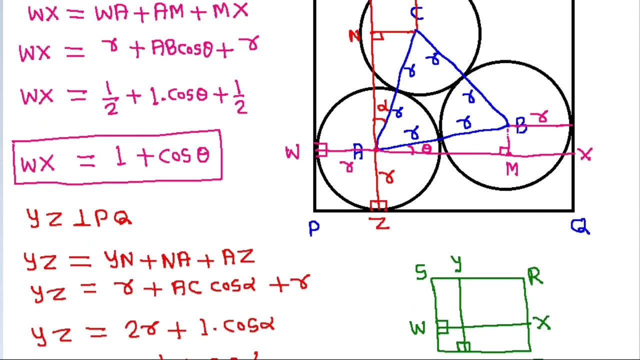 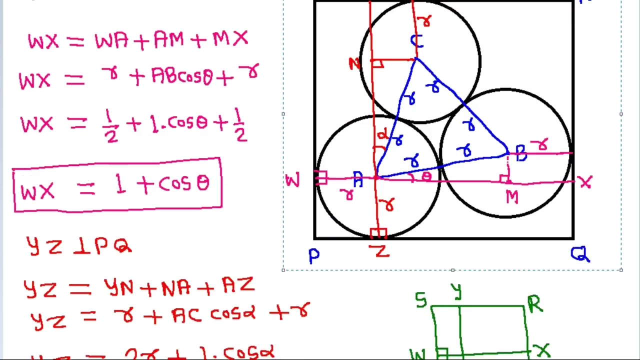 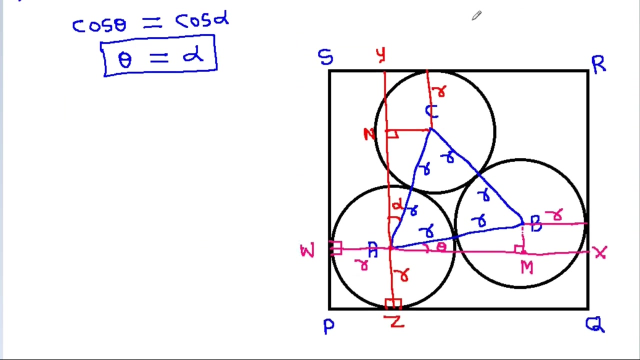 So cos theta is equal to cos alpha, That means theta will be equal to alpha. And in triangle ABC, A, B, C. AB is equal to BC, that is equal to CA, so ABC, it will be equinatural. 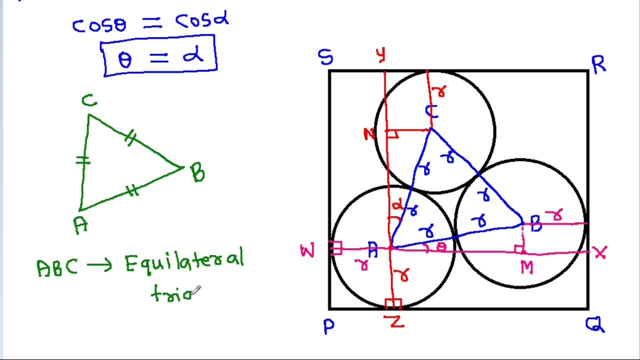 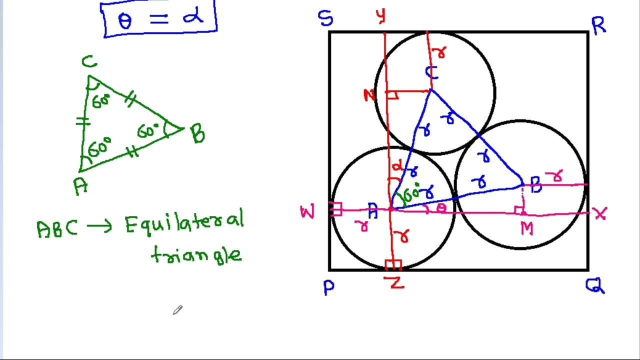 okay, Okay, Triangle. so these angles will be 60 degree. this angle is 60 degree and angle Y A X it will be 90 degree, and angle Y A X is alpha plus 60 degree, plus theta, that is. 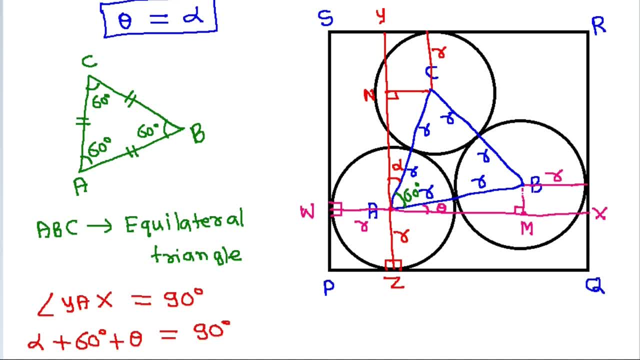 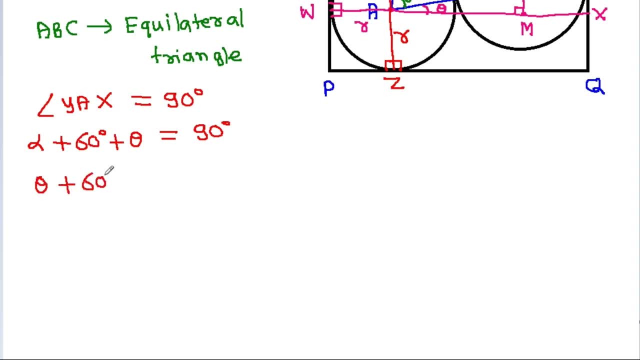 90 degree and alpha is equal to theta plus 60 degree plus theta is equal to 90 degree, and 2 theta plus 60 degree is equal to 90 degree. so 2 theta will be equal to 30 degree. 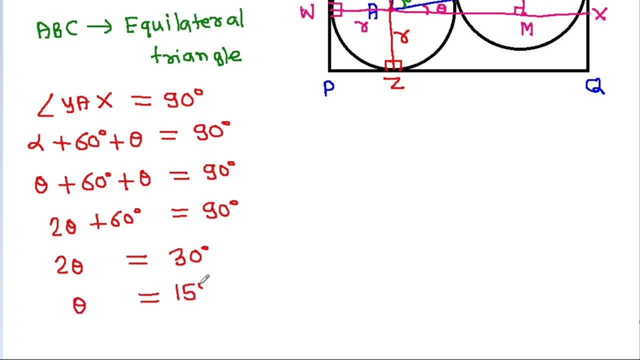 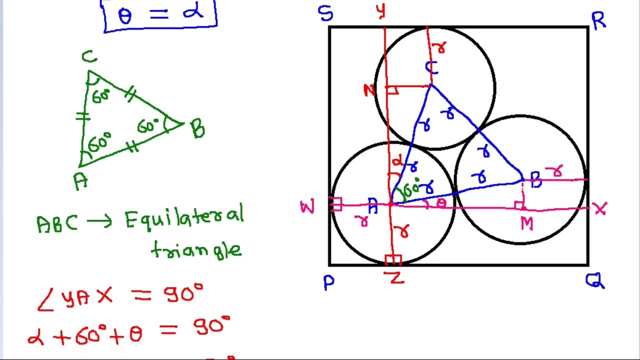 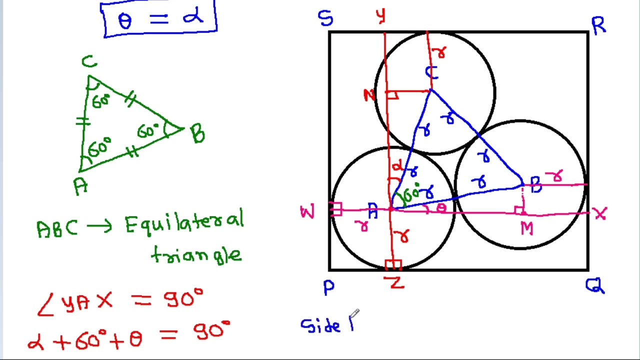 and theta will be equal to 15 degree. And here see, this angle is 90 degree. This angle is 90 degree. This angle is 90 degree. This angle is not 90 degree. So also here, ula is equal to cat. 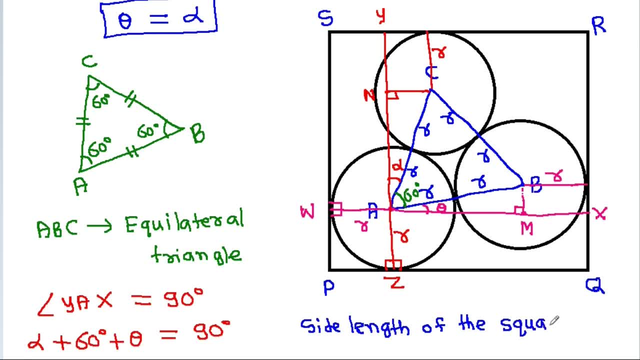 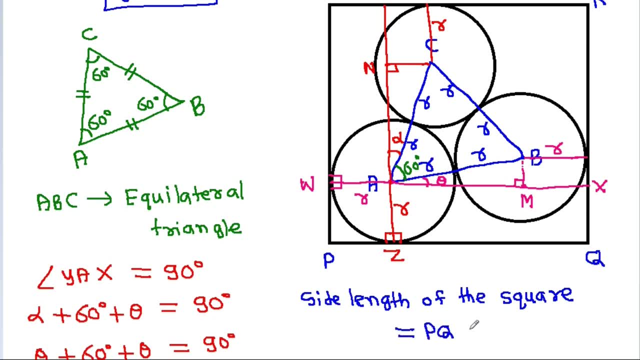 Sobrar Wao Sa has coincident here. So every many degrees. So breakup now causes coronary valance. So these angles are in one side and the other side is counter clockwise. So inуж meters away from there, Thats equal to, And this angle is a circular resistance. 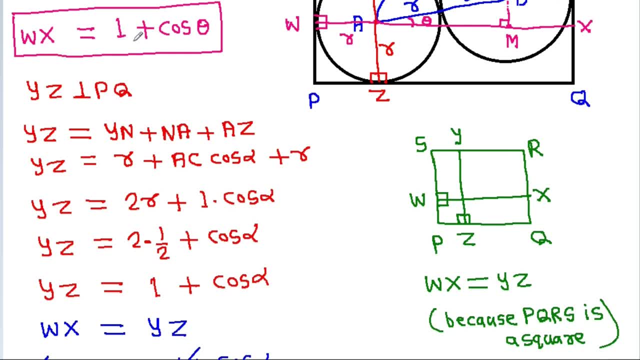 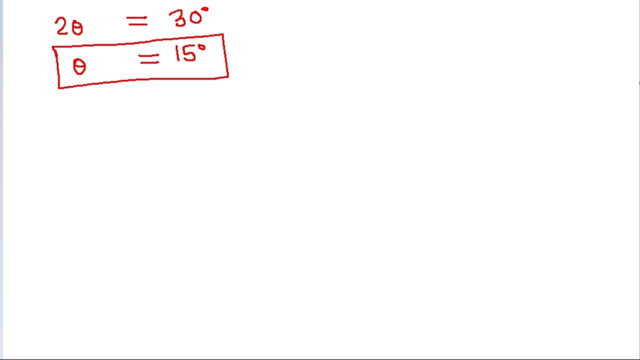 So. so there is no direct descent of PQ and PQ and so, because of tropical managing of waves, So 1 plus cos, theta side net of D square, it is equal to Wx, that is equal to 1 plus cos.